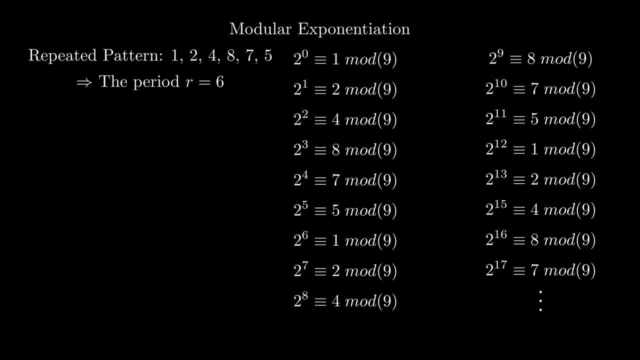 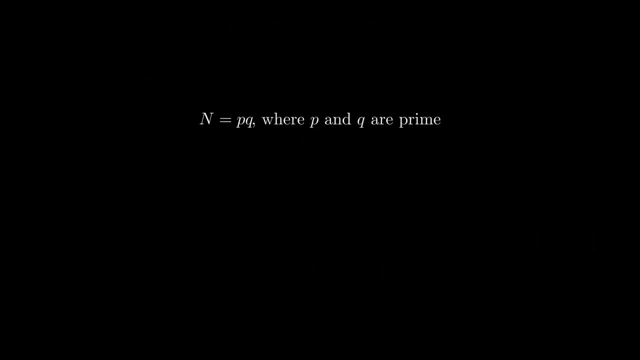 of 0 is congruent to 1 mod n, so we need to keep increasing the power until we get back to 1.. If we are able to find the period, we can use some number theory to find the prime factors. If we have a number n which is equal to the product of two prime numbers, then we can. 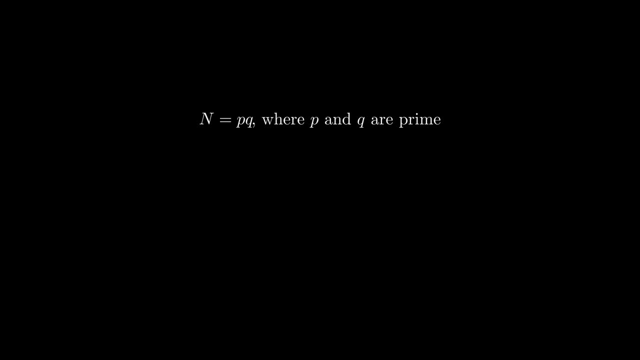 use the prime numbers p and q. If we pick a number a where the gcd of a and n is equal to 1, so they share no common factors- and we find the period of a to the x mod n, then if we get a good approximation for R, the gcd of a to the power of R divided by 2 minus. 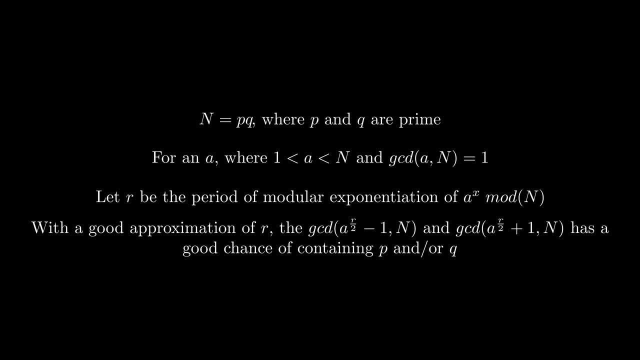 1 and n, and the gcd of a to the power of n divided by 2 plus 1 and n, has a good chance of containing the factors of n. Let's go through the steps in finding the period of modular exponentiation For this. 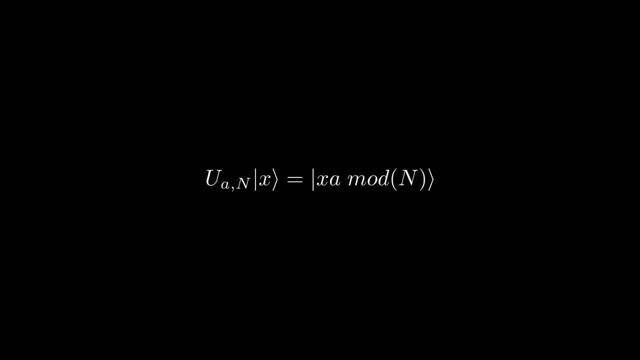 we need to use this gate- let's call it u, which transforms the state x to the state mod n. If we apply this gate to the one state multiple times, we can get powers of a in mod n. How we construct this gate is outside the scope of this course. See the problem set for resources. 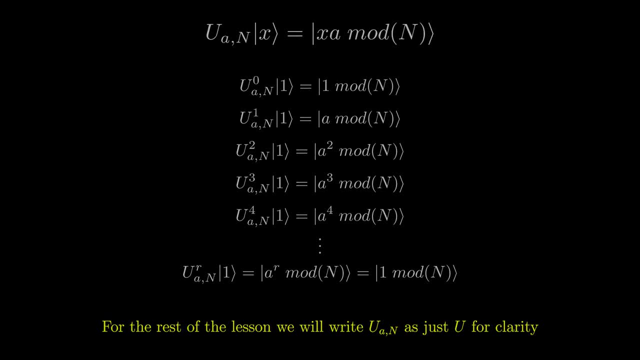 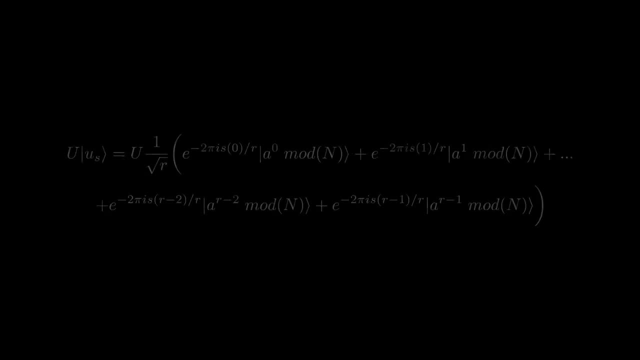 on how we can construct this gate. Let's consider this state u s. If we apply a u gate to the state, it gives us this state. Looking at the a to the r mod n, we can change this to a to the 0 mod n, since they are both. 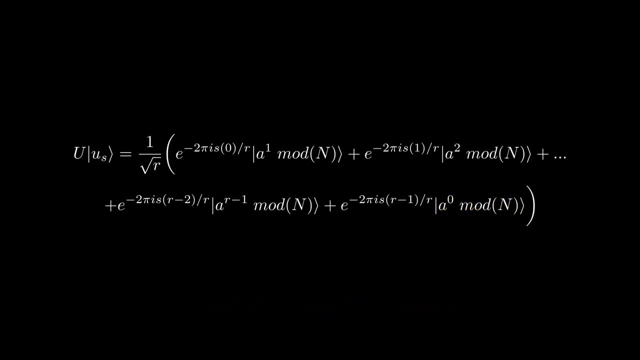 1. If we multiply the right hand side by 1, or e to the 2 pi i s over r times, e to the negative 2 pi i s over r, we get this state. We can change the e to the negative 2 pi i. 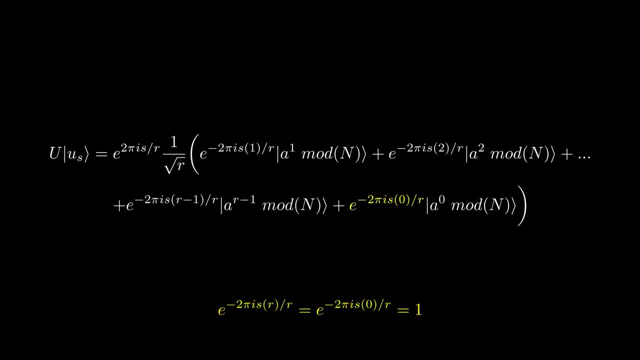 s r over r to e, to the negative 2 pi i: 0 over r, since they are both equal to 1.. Now, as you can see, this whole state becomes the u s state. This means that the u s state. 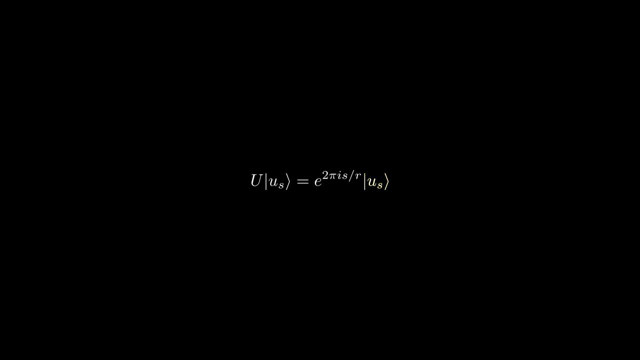 is an eigenvector of the? u gate with an eigenvalue of e to the power of 2 pi i over r. This means that if we can construct the? u s state, we can use the quantum phase estimation algorithm to get the value of s over r. It turns out that it is far easier to construct. 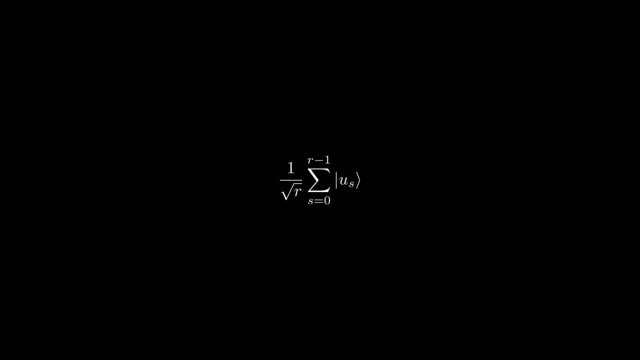 the equal superposition of all of the u s states. What this becomes is 1 mod n. In the problem set for this lesson we will prove this result. We can construct the 1 mod n by applying a knot. Here is the circuit for the algorithm. Looking at it, this is just the quantum phase estimation. 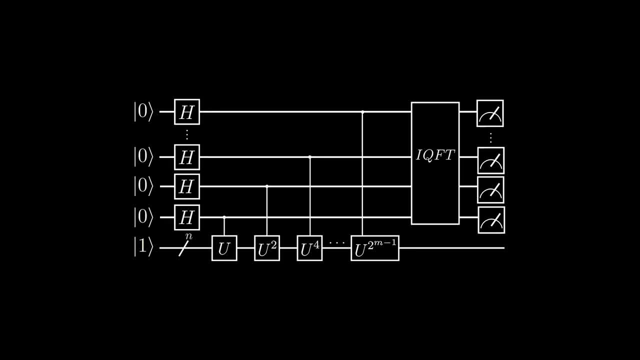 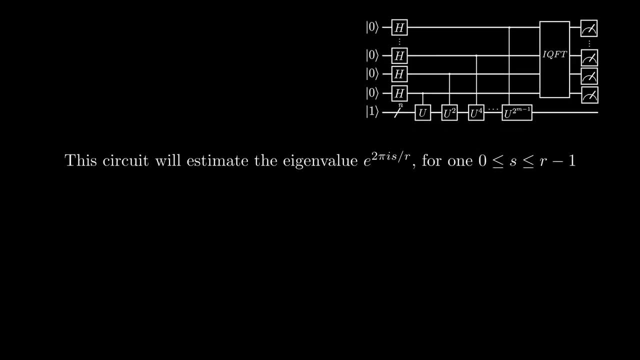 circuit. As you can see, we now know that 1 is an eigenvector of the u gate, so we are using this to estimate the eigenvalue e to the power of 2 pi i s over r, where s is an integer from 0 to r minus 1.. This is because our eigenvector 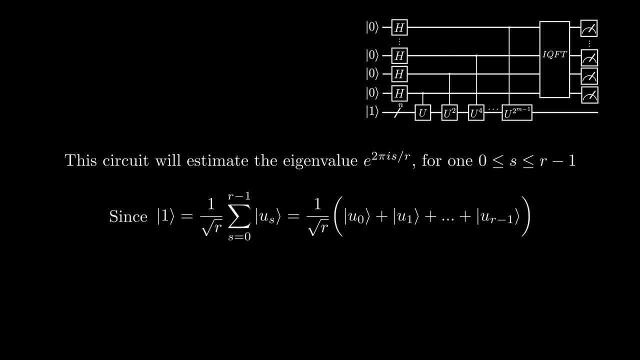 1, mod n is equal to 1 over root r times. the sum from s equals 0 to r minus 1, of u s. So we will get the eigenvalue e to the power of 2 pi i s over r for one value. 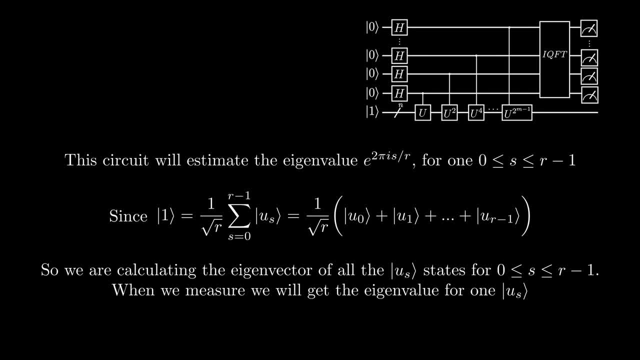 1. of s. So when we measure the qubits, we will get the eigenvalue of 1 of the us's, which means that we will get s over r for 1s from 0 to r-1.. If we happen to get 0 as our eigenvalue, 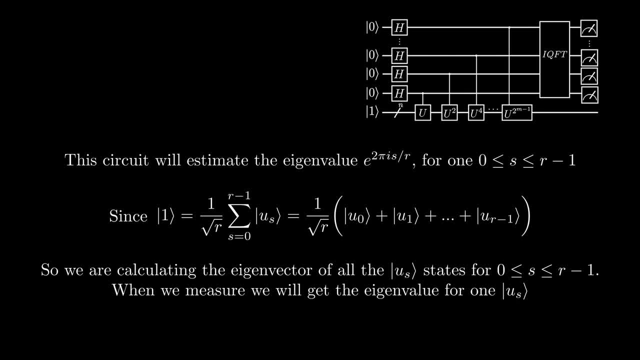 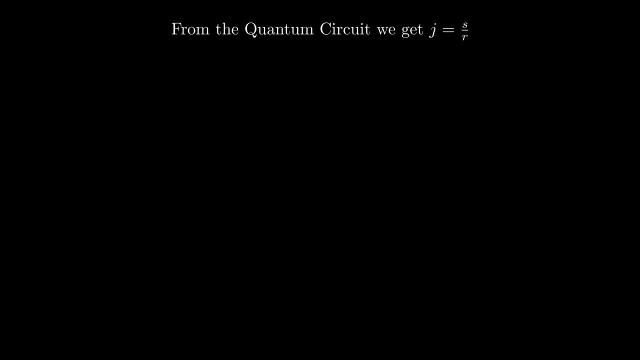 so s equals 0, then we repeat the circuit so we can get an eigenvalue that is non-zero. Now we have a decimal number, j, which is equal to s over r. That is the quantum part of the algorithm done. Now we estimate the values of s and r by using a technique called continued. 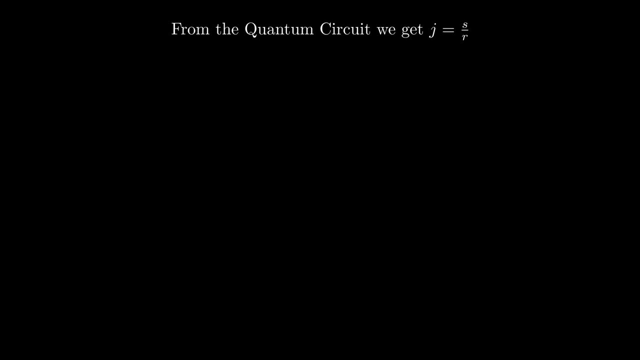 fractions. Here is an example with the decimal 0.312.. We start by writing it as a fraction, then we flip the fraction, We continue this process until we have the number 1 in the numerator. By representing a decimal in this way, we can approximate its value with a fraction. 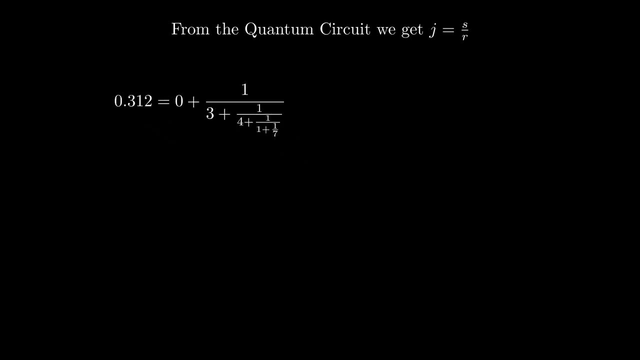 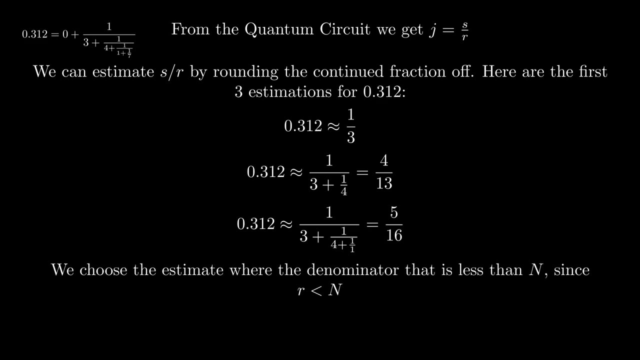 by rounding off the continued fraction. Here are the first three approximations for the decimal 0.312.. To approximate s over r, we find an approximation where the denominator is less than n, since the period r must be less than n. If r is odd, then we repeat the algorithm and get a new value of r. 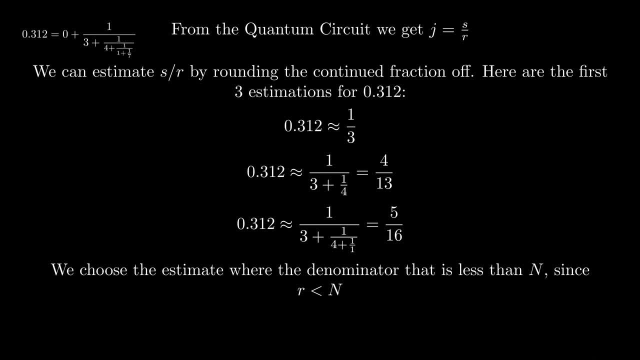 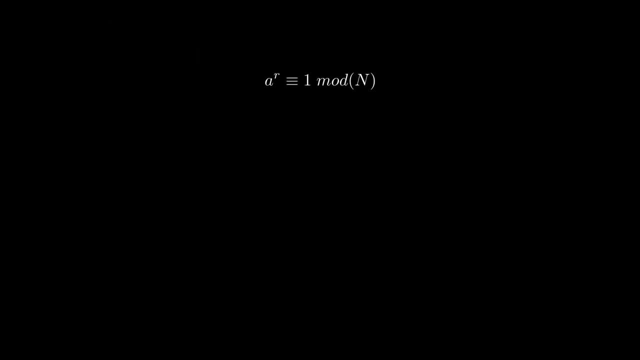 Now that we have a value for r, we can use this to find the factors of n. We know that a to the r is congruent to 1 mod n. so a to the r minus 1 is congruent to 0 mod n. This 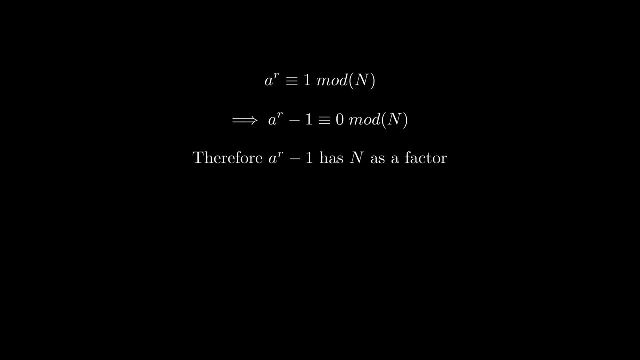 means that a to the power of r minus 1 has a factor of n, since when we divide it by n, we get 0 remainder. If we factor a to the power of r minus 1, with a difference of 2, then we get this. From this we can see that if we calculate the GCD of a to the power of r over 2, 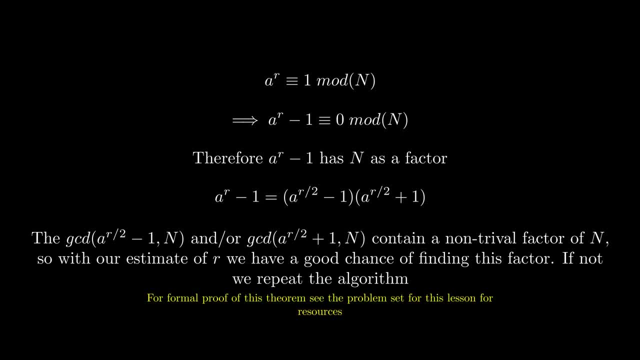 minus 1, n and the GCD of a to the power of r over 2 plus 1 and n. with our approximation of r, we have a good chance of them being one of the factors. This allows us to find p and q. 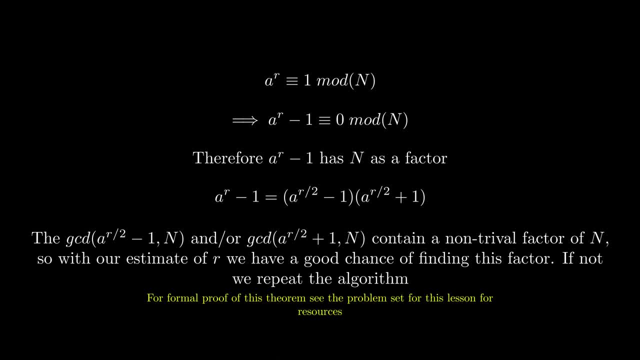 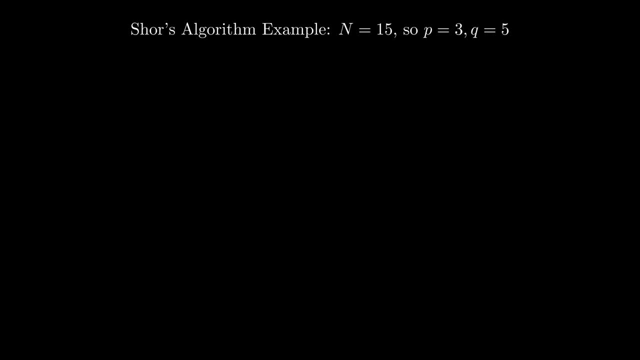 Let's go through a quick example with n equal to 15. So p is 3 and q is 5.. In step 1, we choose an a which is relatively prime to 15. Let's choose a equals 7.. Now, in step 2,. 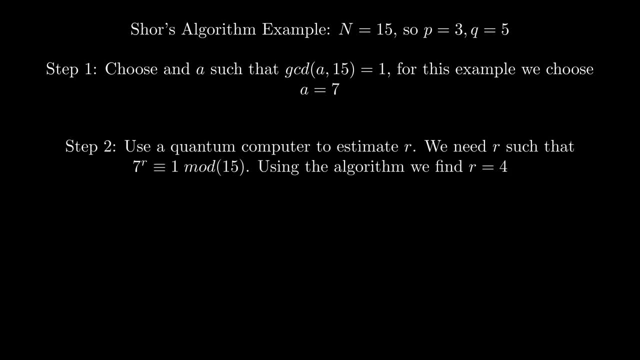 we use the quantum part of Shaw's algorithm to find the period, or r. So we need to find r such that 7 to the power of r is congruent to 1 mod 15.. By using the quantum part of Shaw's algorithm, we find that r is equal to 4.. Now we calculate the GCD of 7 to the power of 4 over 2.